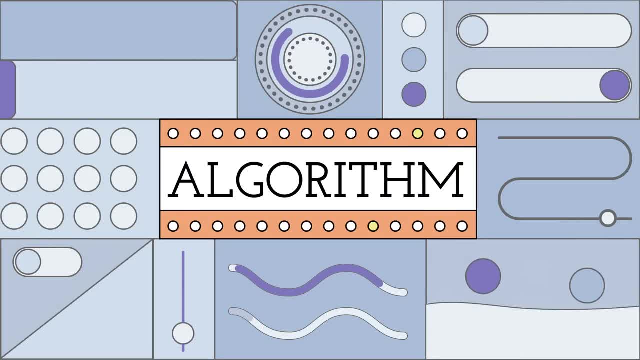 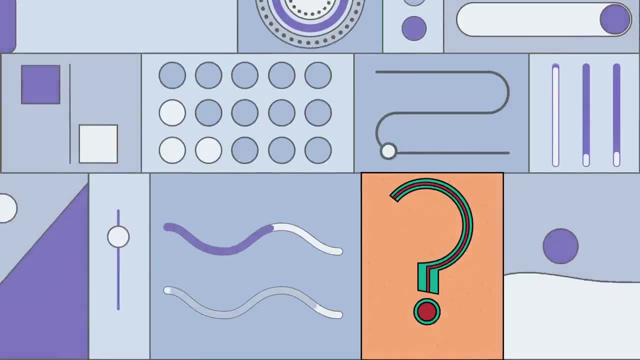 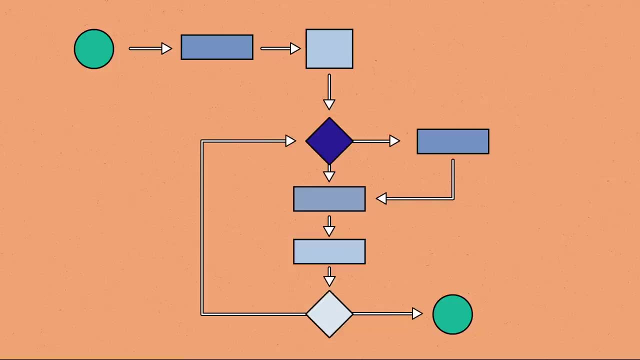 You may have heard the term algorithm recently, whether it was online or maybe in some conversation about technology. It's a word that gets thrown around a lot, but what exactly does it mean? Well, simply put, an algorithm is a set of steps used to complete a specific task. They're the building blocks for 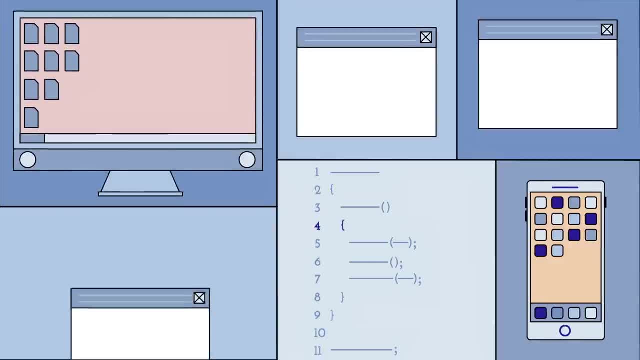 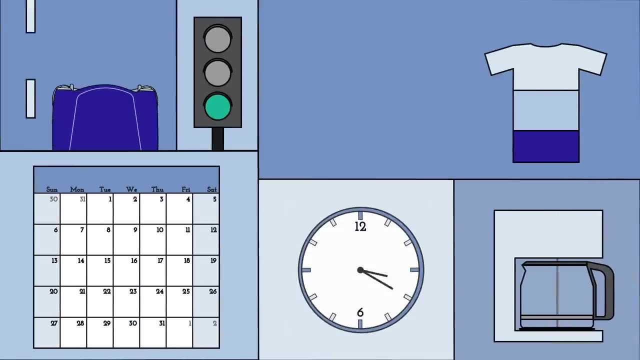 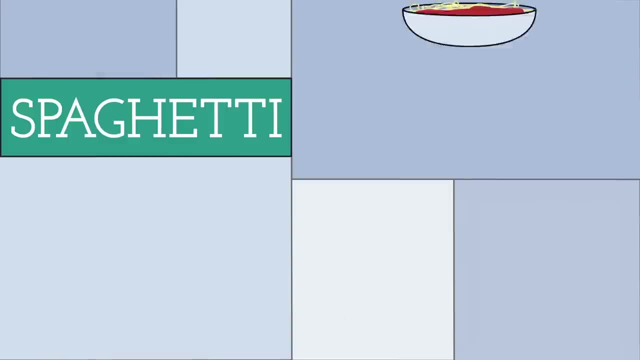 programming, and they allow things like computers, smartphones and websites to function and make decisions. But in addition to being used by technology, a lot of things we do on a daily basis are also similar to algorithms. Let's say, you want to make some spaghetti. In order to do this successfully, there's a certain 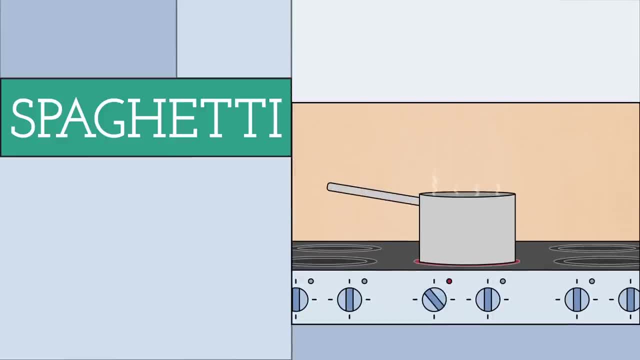 set of steps you need to follow in a particular order. First, you need to boil a pot of water. Once it's boiling, you then add the spaghetti and cook it for a set amount of time, stirring occasionally. Once it's finished, you drain the water. 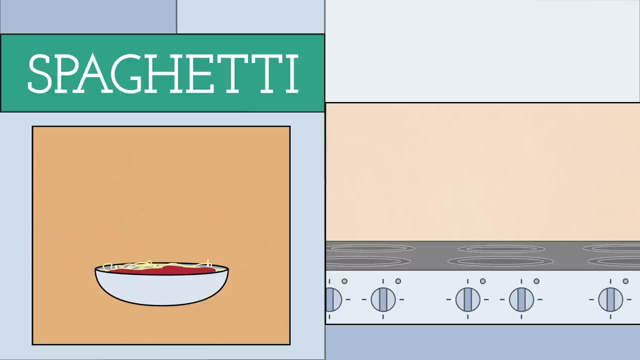 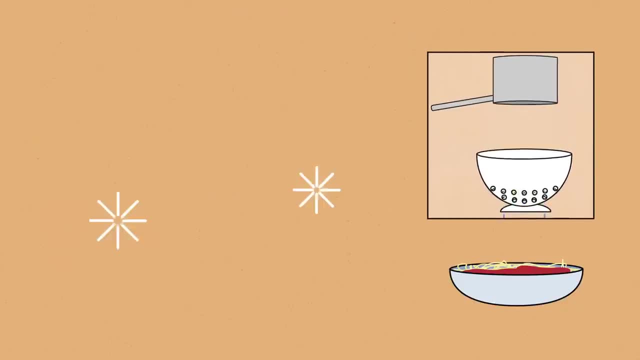 and then it's ready to be served with a sauce of your choice. That entire process is actually an algorithm. Because you followed those steps in that order, you reached your desired outcome: a delicious pasta dish. But if you were to make a mistake, say over or under cooking your noodles, it probably wouldn't be as good. 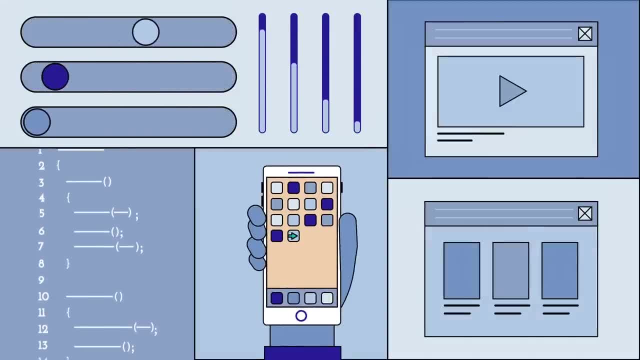 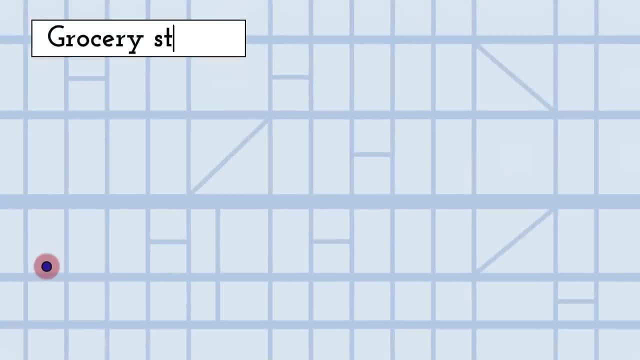 Programs work in a similar way. Their code is made up of algorithms telling them what to do. Let's say that we want to use a navigation app to get directions. When we punch in a destination, the app uses an algorithm to look at the various available routes. Next, it uses a different algorithm to 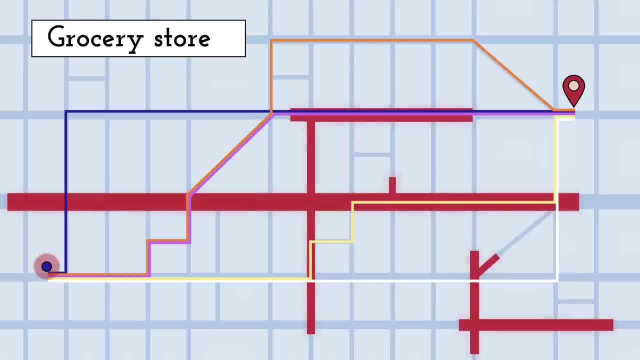 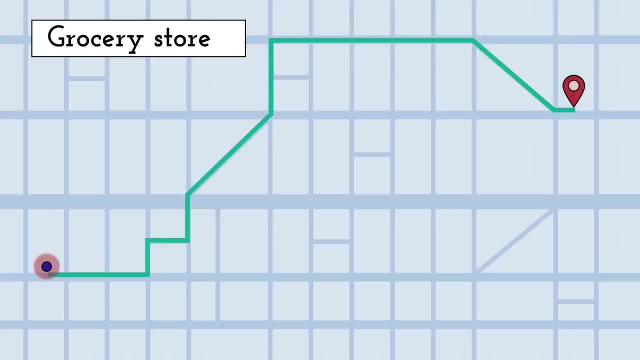 check the current traffic, And then a third one takes that information and calculates the best available route. All of these algorithms are built right into the app's code. If there were any kind of error in that code, the app wouldn't be able to follow these algorithms correctly, meaning you wouldn't receive. 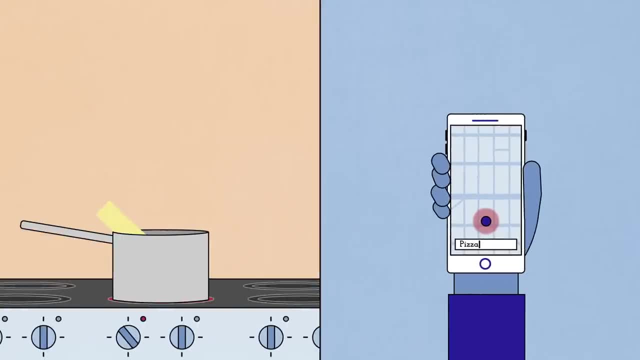 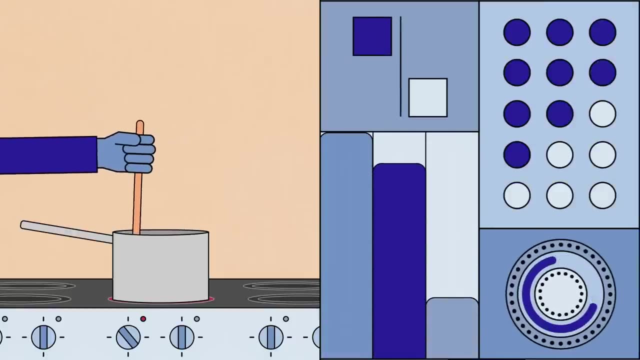 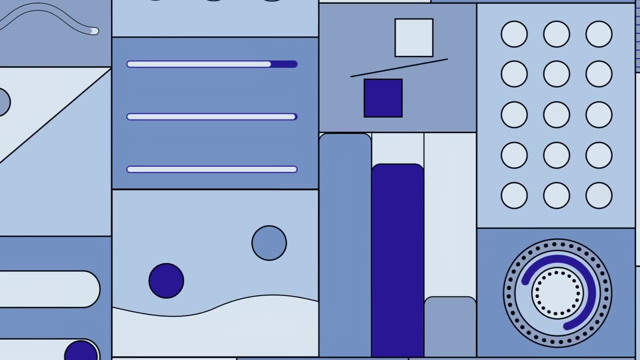 your directions. Both of these examples show how both humans and computers can use algorithms to perform everyday tasks. The difference is that computers can use algorithms and calculate things better, faster and more efficiently than we can. Technology is only going to continue to evolve and get even better.